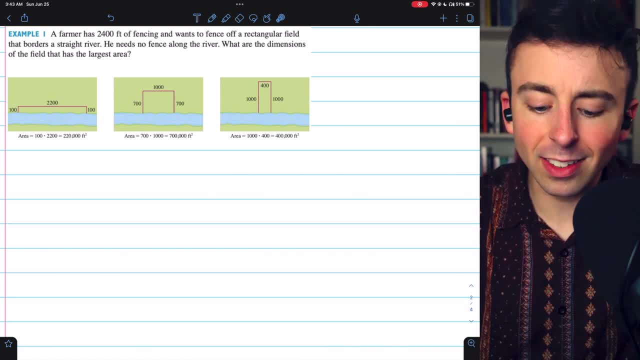 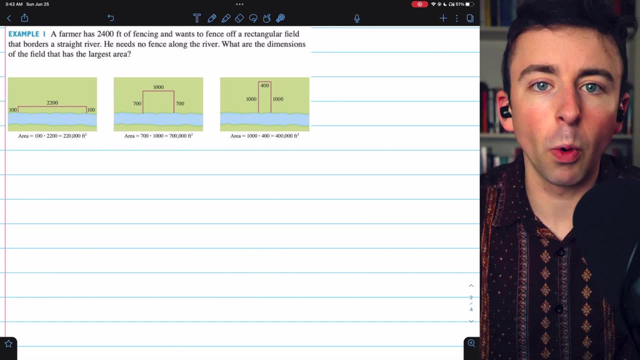 we also get a small area. If we go for a more balanced approach, though, the area is much larger. So there's got to be some optimal point, some optimal dimensions for this fenced-off area, giving us a maximum area, And that's what we're looking for. We'll begin with a sketch of the 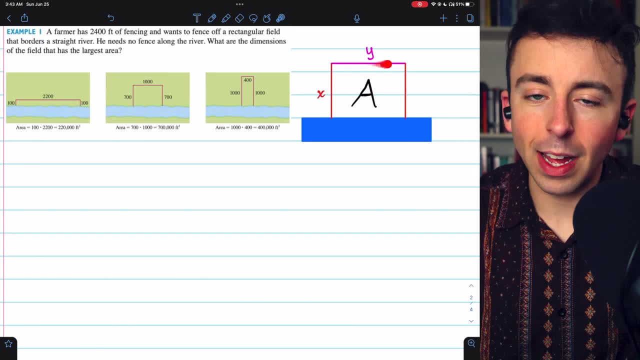 situation. We have this river and then we have our fenced-off area. We'll say that the side of the river is a little bit smaller than the other side. We'll say that the side of the river is a little bit smaller than the other side. We'll say that the side of the river is a little bit. 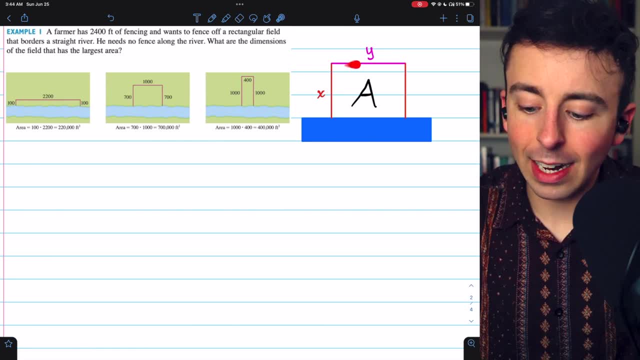 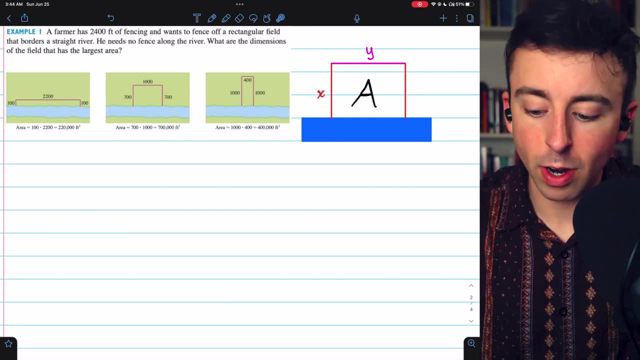 smaller than the other side. We'll say that the side of the river is a little bit longer than the other side. The other side of our rectangle, opposite the river side, has a length of y, And then the other two sides that we need both have a length of x. We, of course, are trying to maximize the area. 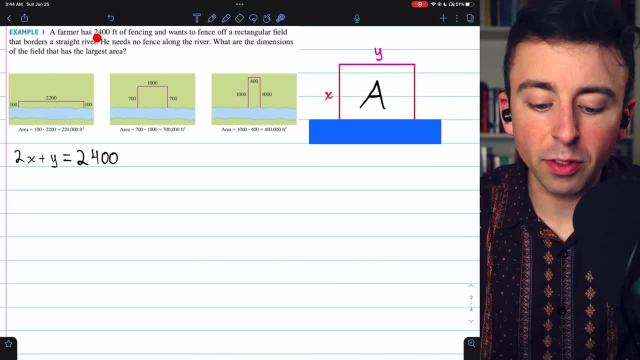 of this rectangle. We do have some given information, which is that we have 2400 feet of fencing. So x plus x plus y or 2x plus y will have to equal 2400.. That's all the fencing we have. 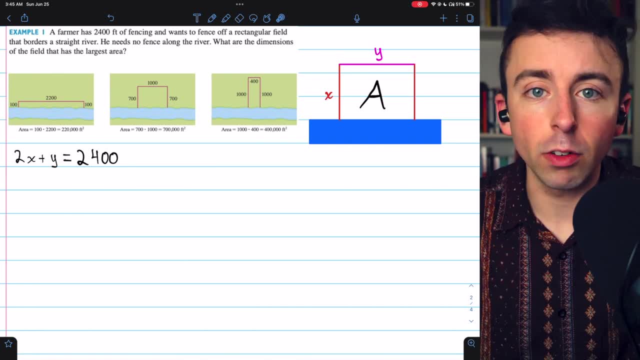 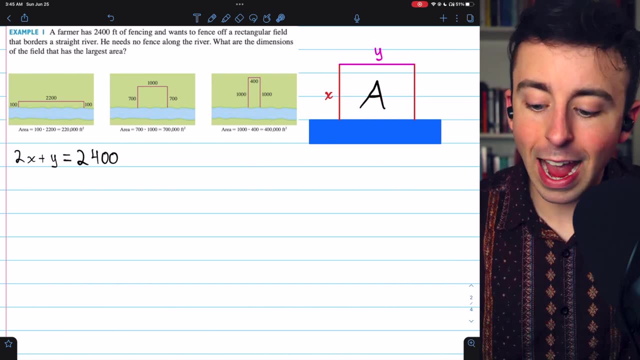 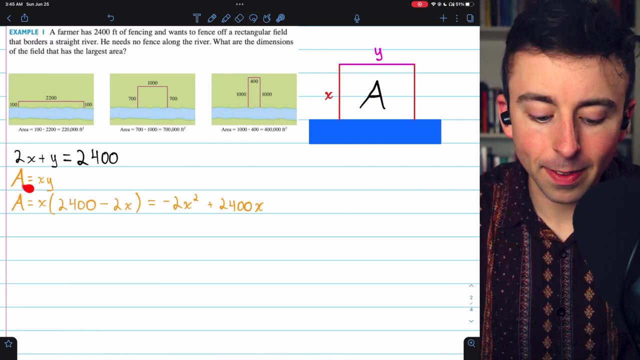 Now we can move on to the primary equation. Let's write an equation for the quantity that we're trying to optimize. we're trying to maximize area, so we'll write an equation for that. the area of this rectangle is, of course, just X times Y, so that's our primary equation: a equals X, Y. again, though, we've got two. 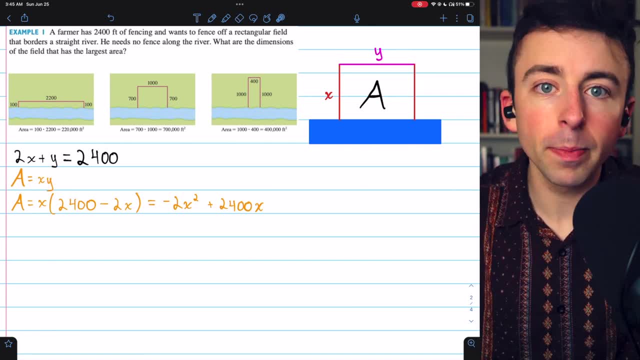 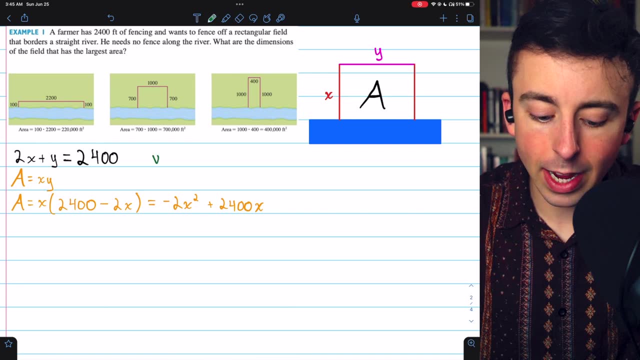 variables. here we need an equation in terms of a single variable. we can fix that pretty easily. this is step three, by going back to our secondary equation and solving for Y. Y is equal to 2400 minus 2x, and then we can plug that in for y in. 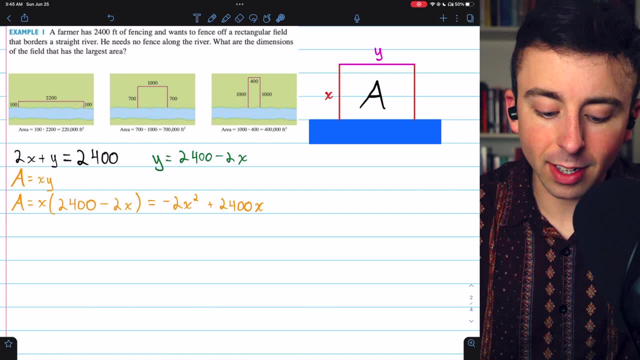 our area equation to find that the area is equal to X times 2400 minus two X, which is the same as negative 2x squared plus 2400 X. now we have a primary equation in terms of a single variable. the next step is to establish the. 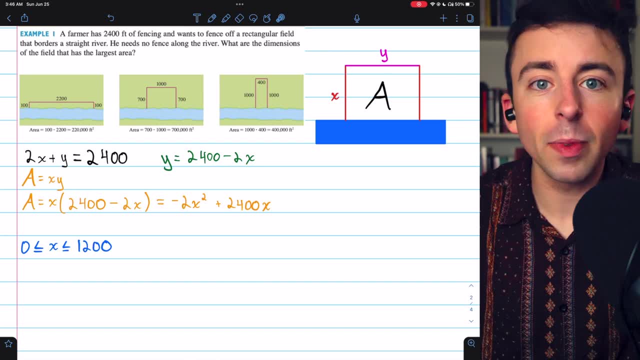 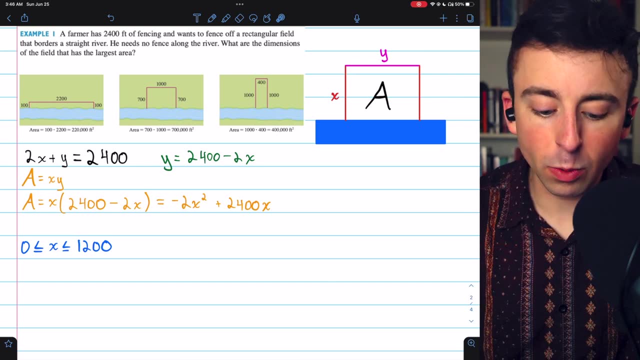 feasible domain. in this case X has to be between 0 and 1200- we obviously can't have a Ihnen negative dimension on our rectangle- and x has to be less than or equal to 1200, because the amount of fencing we have is 2400 and there's two copies of x in our design, so x can't exceed 1200. we don't.